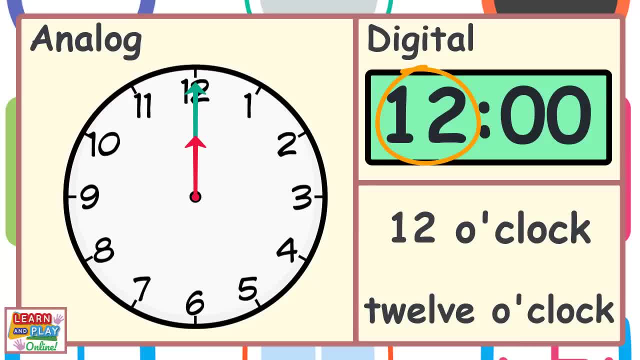 The digits on the left will tell us the hour that we're in. The digits on the right tell us how many minutes have passed the hour. The time on both the analogue clock and the digital clock both say 12 o'clock. Since there are 60 minutes in one hour, let's have a look at what happens when the minute 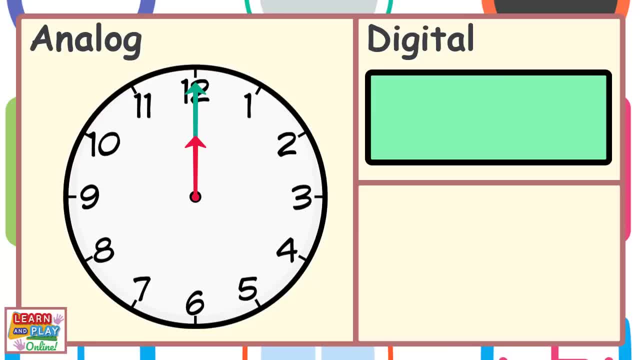 hand moves clockwise around the clock. The minute hand is pointing to the 12, so it is something o'clock. The hour hand is pointing at the number 1, so the time is 1 o'clock. Let's watch the clock fast forward another 60 minutes. 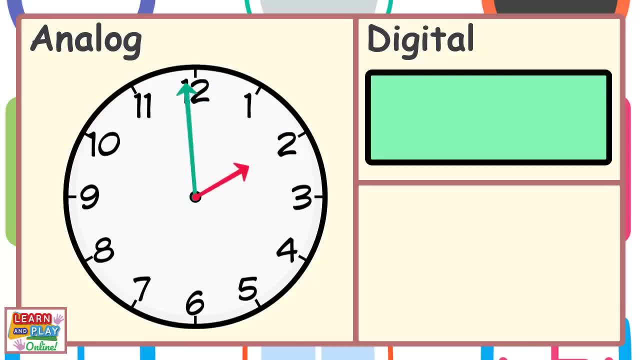 What time is it? It is two o'clock. Try to remember the basics. When the minute hand is pointing at the number 12, it is something o'clock. So then look at the hour hand to tell you what that something o'clock is. 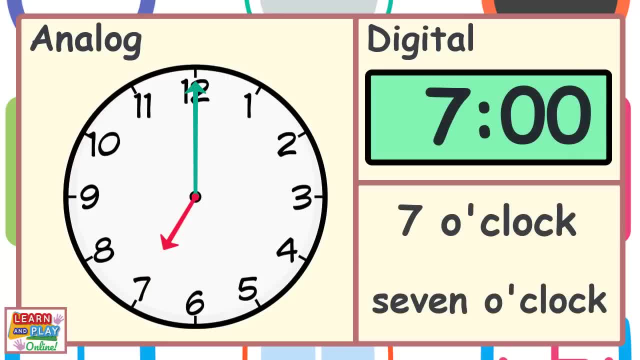 The time is seven o'clock. It is eleven o'clock. The time is three o'clock. It is six o'clock. The time is eight o'clock. The time is seven o'clock. The time is eight o'clock. The time is nine o'clock. 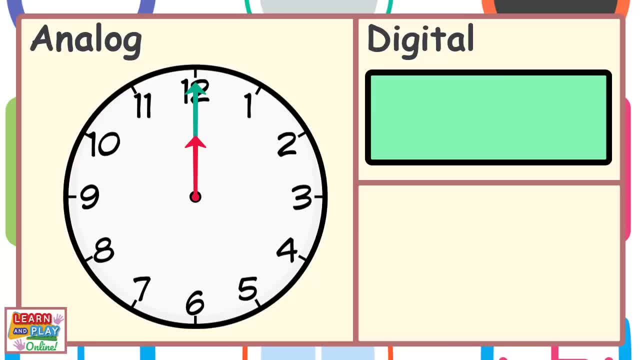 hand moves clockwise around the clock. The minute hand is pointing to 12, so it is something o'clock. The hour hand is pointing at number 1, so the time is 1 o'clock. The hour hand is pointing at the number 1, so the time is 1 o'clock. 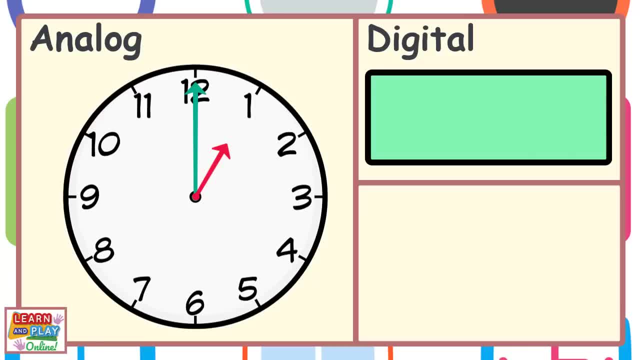 Let's watch the clock fast-forward for another 60 minutes: Fast right-Click, Fast, Right-Click, Fast, Right-Click, Fast, Cubect, Fast-Yaw. What time is it? It is two o'clock. Try to remember the basics. When the minute hand is pointing at the number 12, it is something o'clock. 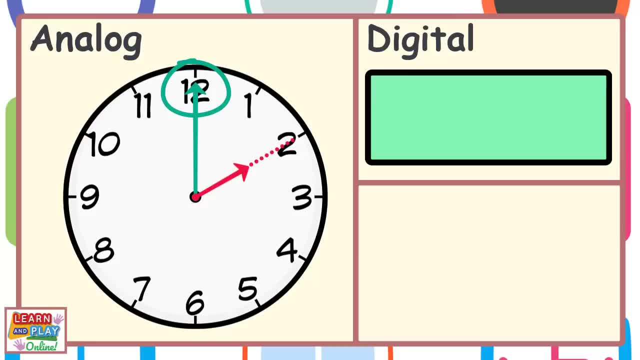 So then, look at the hour hand to tell you what that something o'clock is. The time is seven o'clock. It is eleven o'clock. Okay, The time is three o'clock. It is six o'clock. The time is eight o'clock. 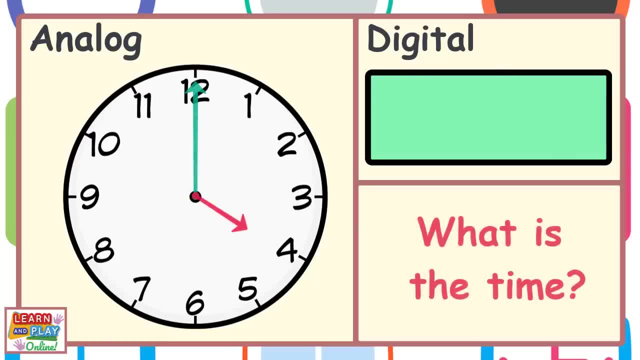 Okay, The time is nine o'clock. It is four o'clock. The time is ten o'clock. It is five o'clock. Okay, The time is seven o'clock. It is five o'clock. The time is six o'clock. It is nine o'clock. 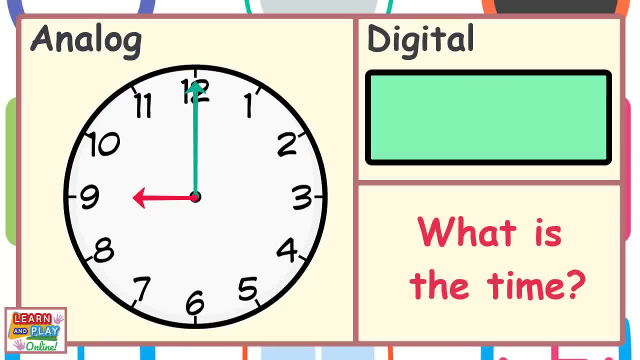 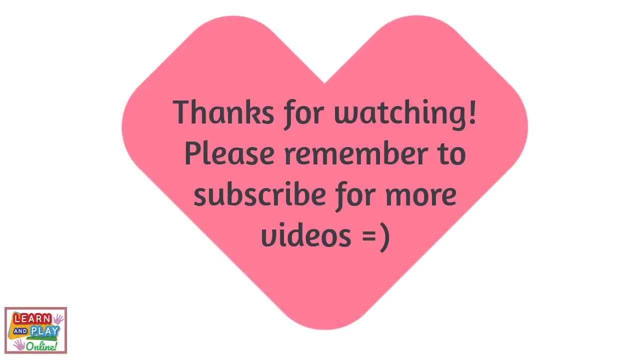 It is seven o'clock. The time is ten o'clock. no, it's nine o'clock, It is nine o'clock. It is six o'clock, It is six o'clock, It is nine o'clock. Okay, guys, Thank you for watching. Bye, Bye, Bye.